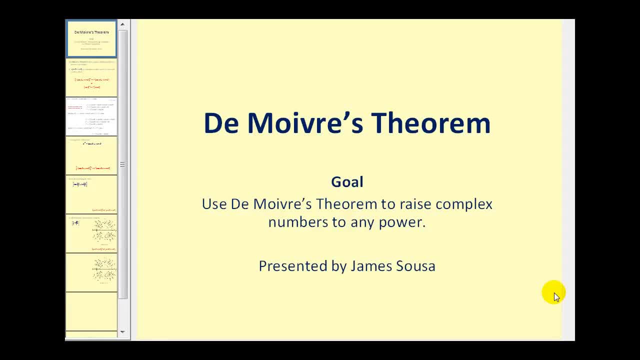 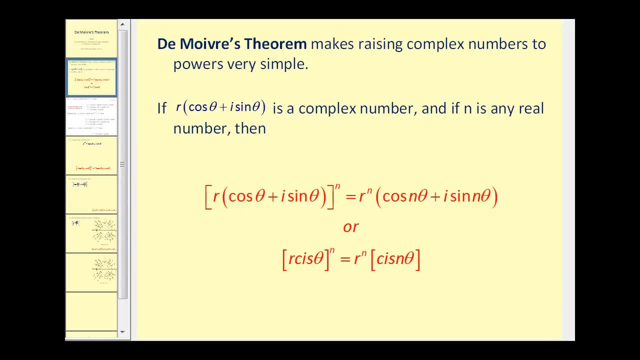 Welcome to a lesson on de Moivre's Theorem. The goal is to use de Moivre's Theorem to raise complex numbers to any power. So de Moivre's Theorem makes raising complex numbers to powers very simple. If r times the quantity cosine, theta plus i sine theta is a complex number, and if n is any real number, 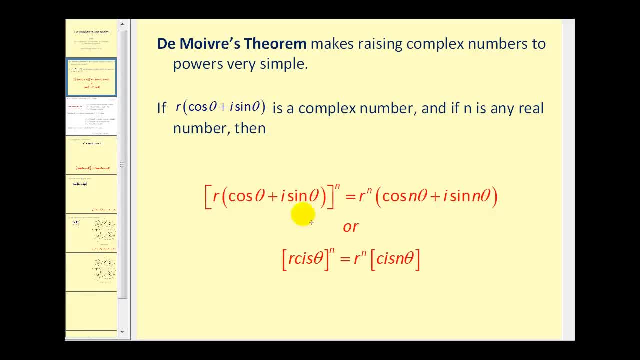 then if we take this complex number and raise it to the power of n, it's equal to r, to the power of n times the quantity cosine n theta plus i sine n theta. So this is a very interesting result. This value of n is used for the power of r. 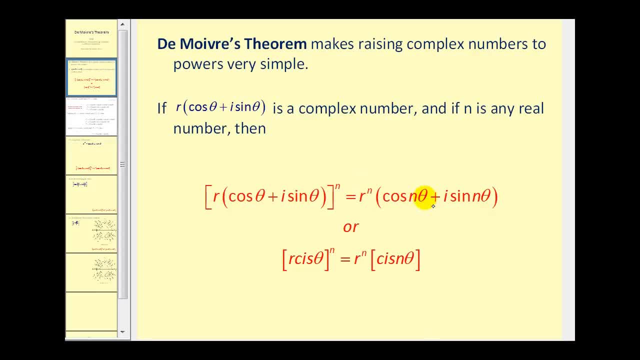 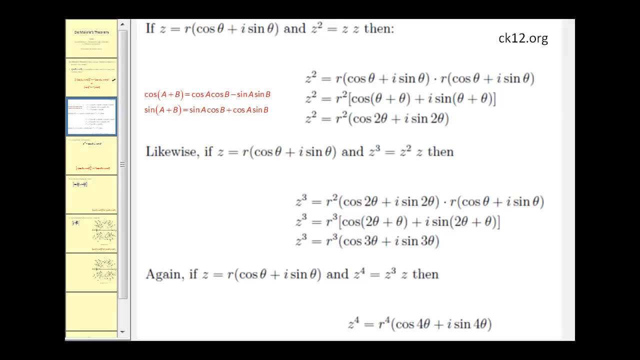 but then it's multiplied by theta to find the new angle, Let's see if we can determine where this formula comes from. One way would be to just start with a complex number in trig form and square it or multiply it by itself, And this will remind you of the product of complex numbers in trig form. 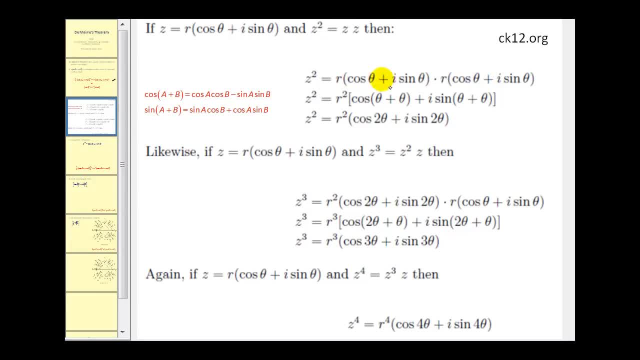 Of course we'd have r times, r, r squared. Then when we multiply this out, it would be the same thing as we saw in the previous video for the product, except now the two angles are the same. So when we apply this, sum identity for cosine, since angle a and angle b would be the same. 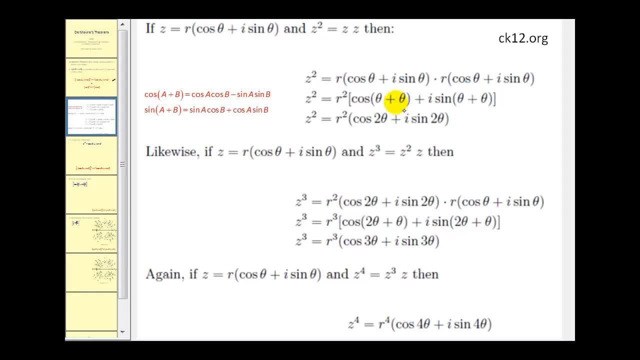 we'd have theta plus theta or two theta, So we'd have the cosine of two theta here And the same for cosine. If we look for the sum identity for sine, since the angles a and b would be the same, we would have the sine of theta plus theta or the sine of two theta. 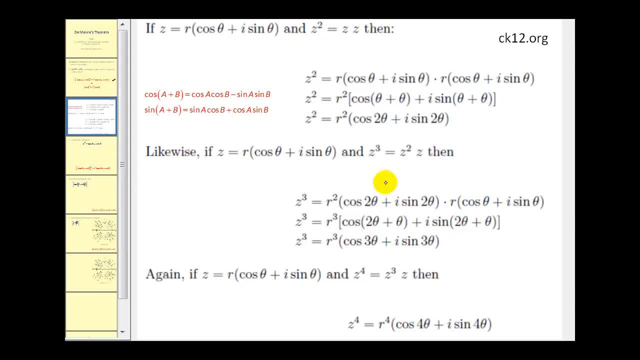 If we take this z squared and multiply it by another z, as we see here, we'll end up with r cubed and then the cosine of three theta plus i sine three theta. So what we're noticing here is that the power that z is raised to is used on the power of r. 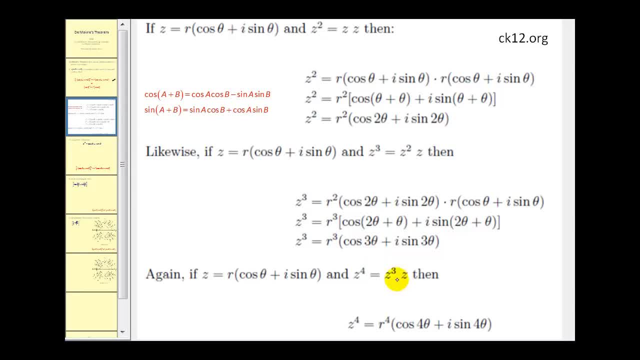 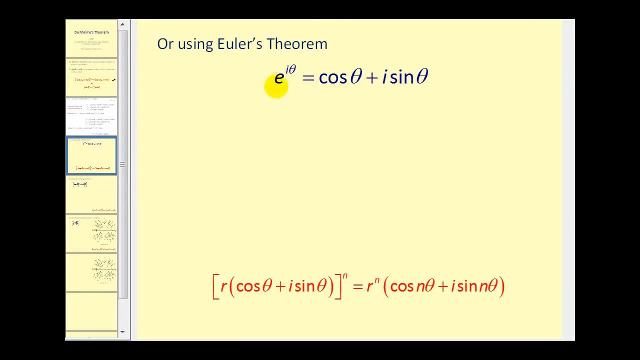 but then it's multiplied by theta to find the new angle, And this pattern does continue. Another way to take a look at this theorem would be to use Euler's theorem, which states: e to the power of i, theta is equal to cosine theta plus i sine theta. 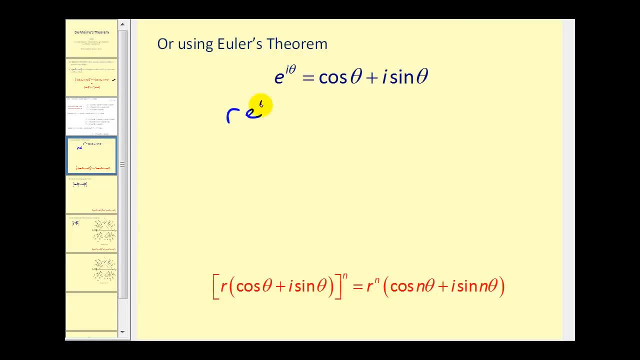 So of course it would follow that r e to the i theta would equal r times cosine, theta plus i sine theta. Before we show the next step, what we should recognize here is that our argument- theta- ends up as the angle for sine and cosine. 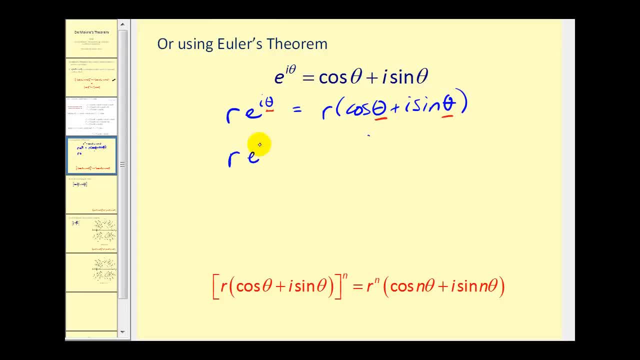 So now, if we take this and raise it to the power of n, this is r to the first power. So we would have r to the n, e to the i n theta. Well, now our argument is n? theta instead of theta. So now we could say this would be equal to r to the n. 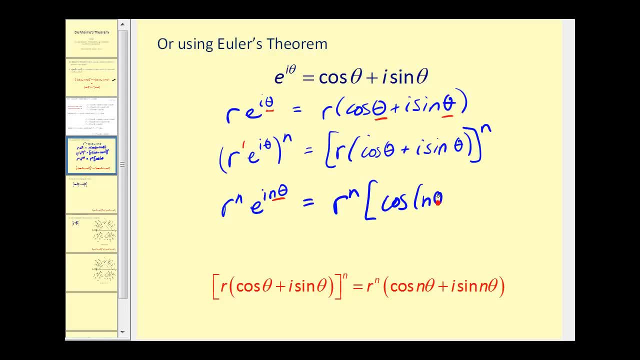 times cosine n theta plus i sine n theta. And this is de Moivre's theorem that states that this, raised to the power of n, is equal to r to the n times the quantity cosine n theta plus i sine n theta. Let's go ahead and see if we can apply this. 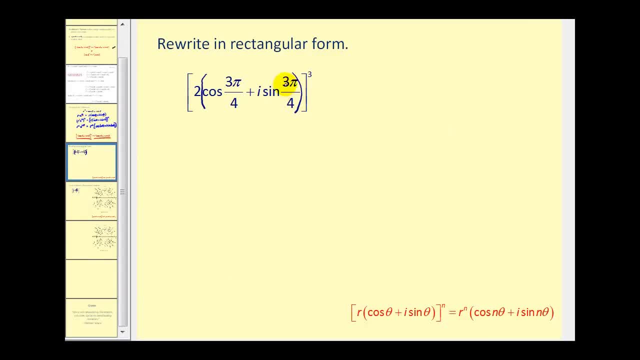 We want to rewrite this in rectangular form, but what we'll do first is evaluate this using de Moivre's theorem and then we'll convert this to rectangular form. So this would be the same as two to the third power times the cosine of three times three, pi over four. 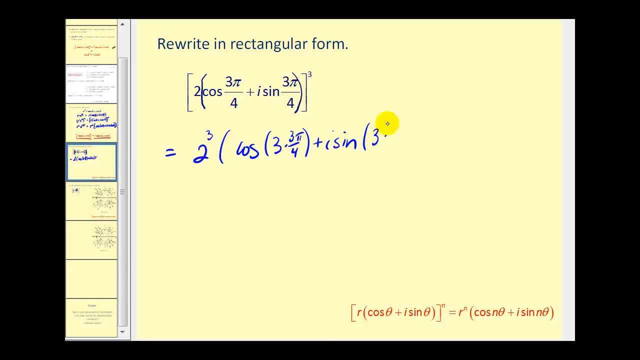 plus i sine of three times three pi over four. So we can see our angle is going to be nine pi fourths. So we'll have eight times cosine nine pi fourths plus i sine nine pi fourths. Let's take a look at the angle: nine pi fourths. 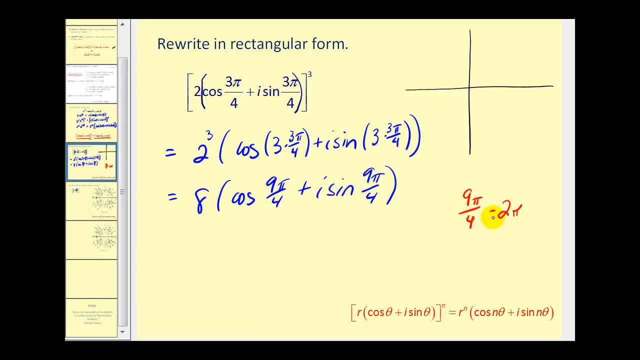 Nine pi fourths would be coterminal with an angle of nine pi fourths minus two pi. Well, two pi is the same as eight pi fourths, So this would equal pi over four. So this angle is coterminal with pi over four. 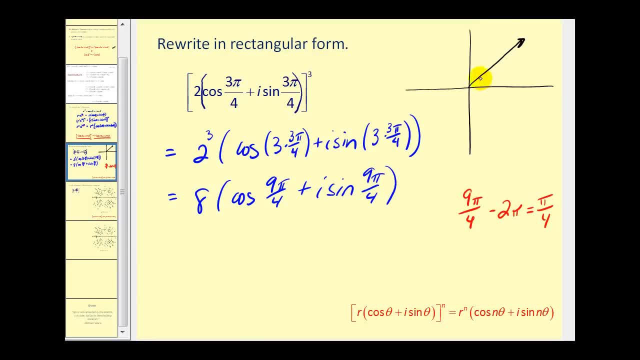 so we'll use that as our reference angle. This is forty-five degrees in the first quadrant, So we have eight times the cosine of nine. pi over four. That would be one over square root two or square root two over two, if we rationalize it. 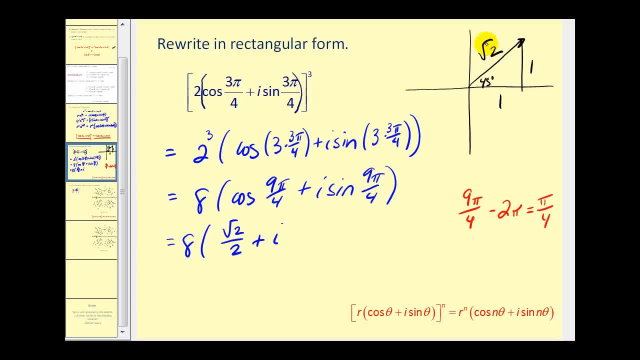 And the same for the sine of nine: pi over four, one over square root two, or rationalized that would be square root two over two. So we have four square root two plus four, i square root two. So you can see if we converted to rectangular form first. 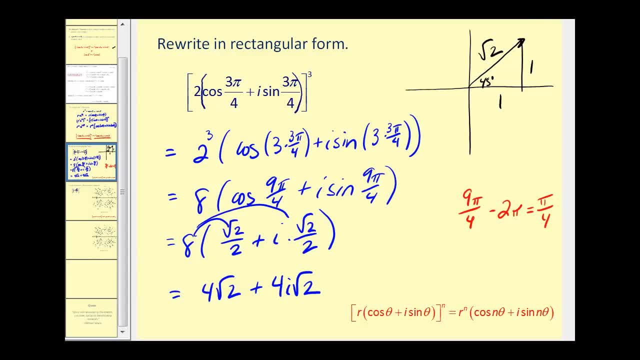 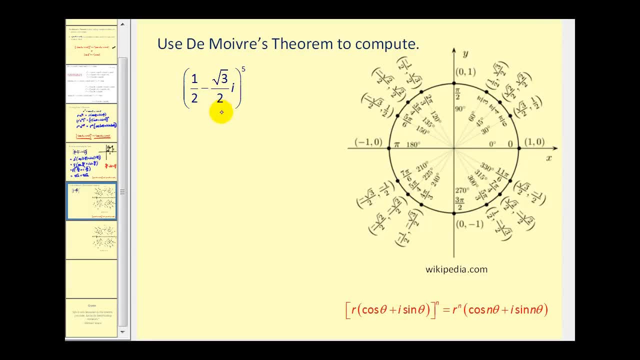 and then tried to cube it. it would be a lot more work. Now we have a complex number in rectangular form, raised to the fifth power. We want to use de Moivre's theorem to compute this, So we'll convert this to trig form. 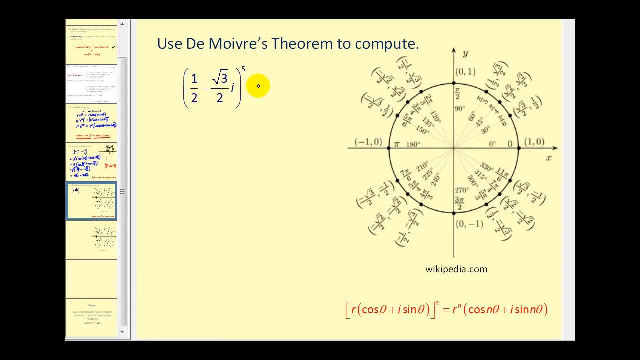 and then we'll raise it to the fifth power. Now I included the unit circle here because it's going to help us dramatically Remember. for this complex number, a is equal to one half and b is equal to negative square root three over two. 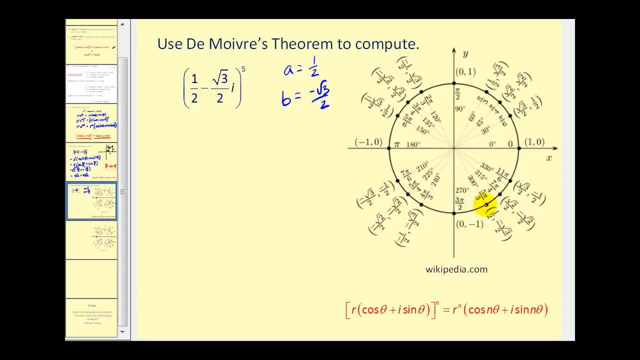 Even though this is the rectangular coordinate plane rather than the polar coordinate plane, we can use this to determine theta. Remember, on the rectangular coordinate plane, a would be x and b would be y. So when x is one half and y is negative square root, three over two. 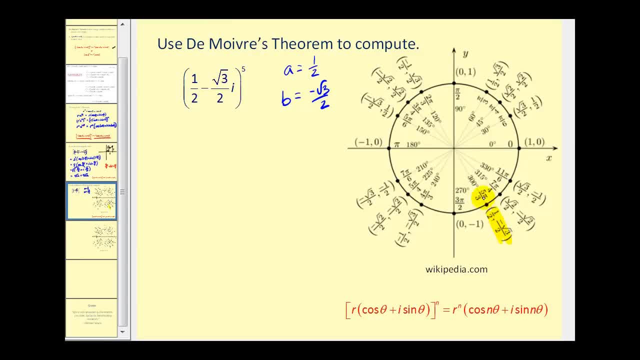 we're actually right here where our angle is three hundred degrees, or five pi over three radians. So that's helpful. Let's use three hundred degrees Next. we're fortunate because that's actually the point on the unit circle. therefore, r would be equal to one. 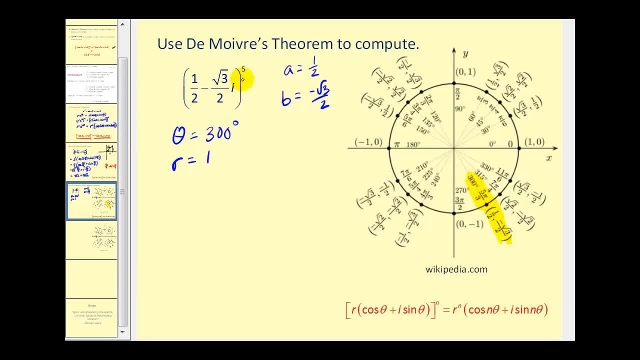 Remember, this is all we need. to write this in trigonometric form, We have one times the cosine of three hundred degrees, plus i sine three hundred degrees, But we're taking this and raising it to the fifth power. So, using de Moivre's theorem, we'll have: 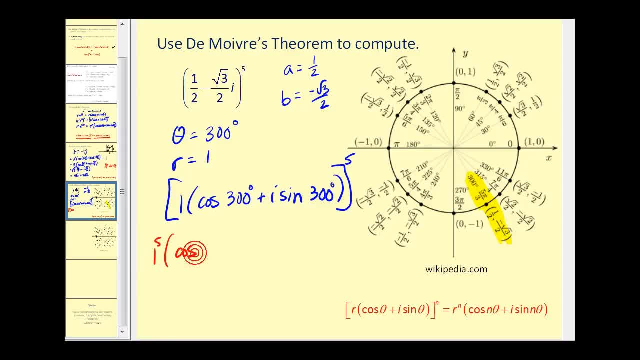 one to the fifth times the cosine of five times three hundred. That's fifteen hundred degrees plus i sine fifteen hundred degrees. Let's go ahead and take a look at fifteen hundred degrees. Let's find the least positive angle that is coterminal to that.